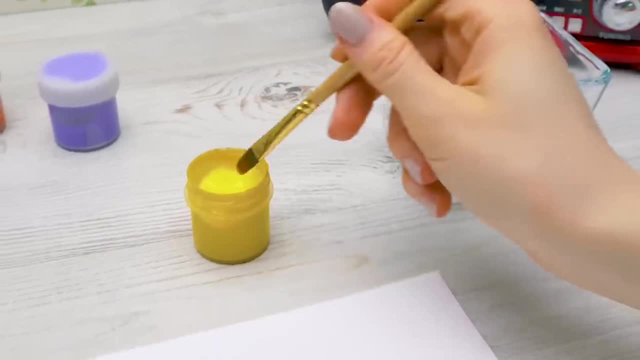 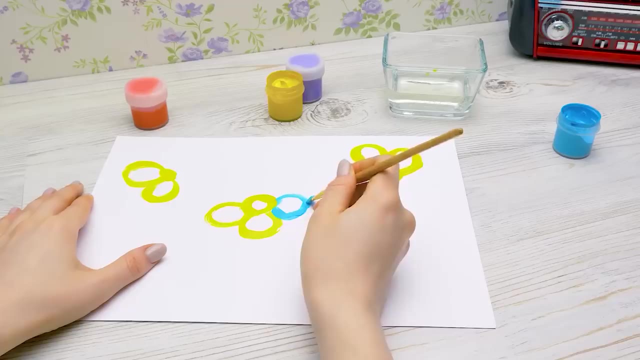 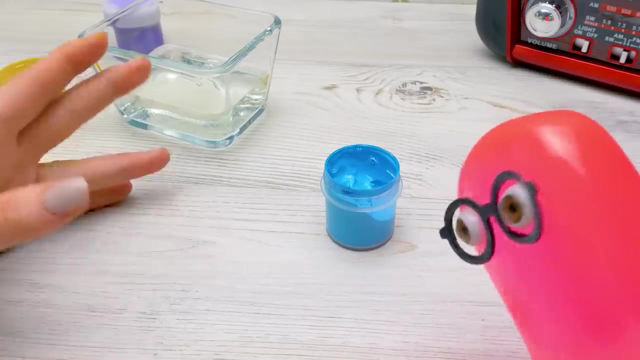 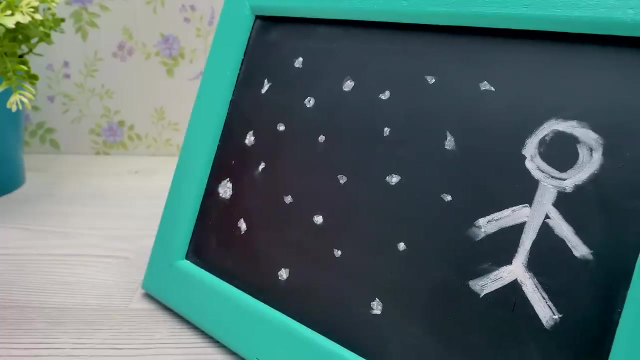 Hmm, Hmm, Hmm, Ta-da. What are you doing? Trolling for a new episode With paint? Yep, What else, Sue my dear baby, let me tell you how YouTube works. This is our wonderful channel, Uh-huh. 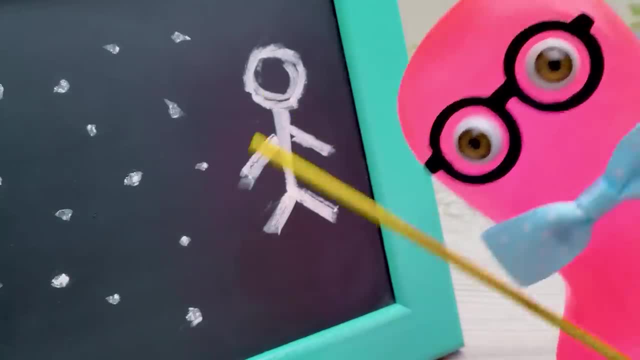 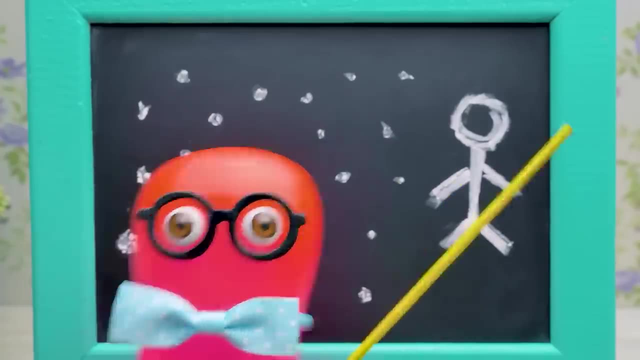 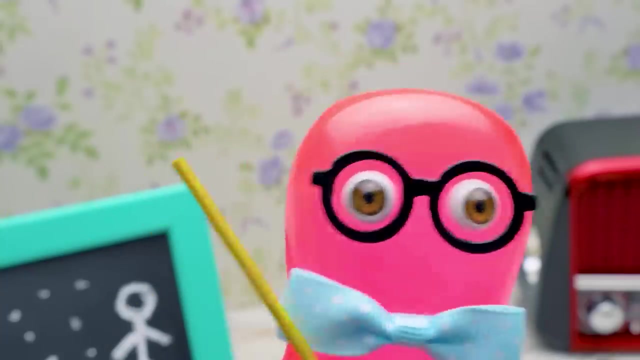 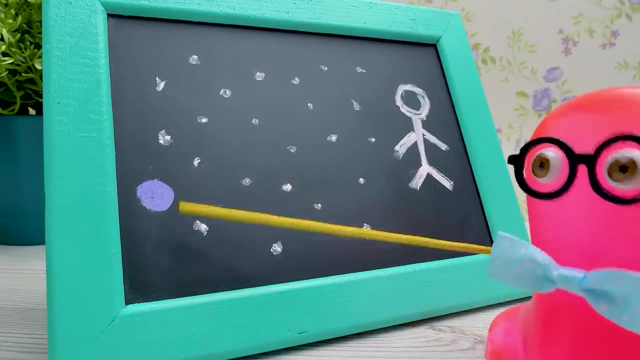 This is our amazing viewer Right, And these are millions of other wonderful channels that are luring our amazing viewer. How to get our amazing viewer to watch our wonderful channel? How Become a purple cow? Huh, Be different from other cows. Do something unique. 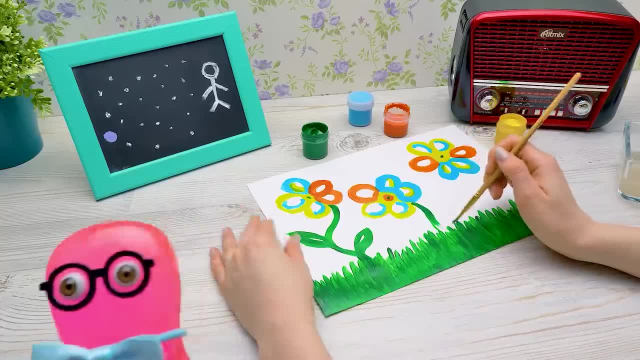 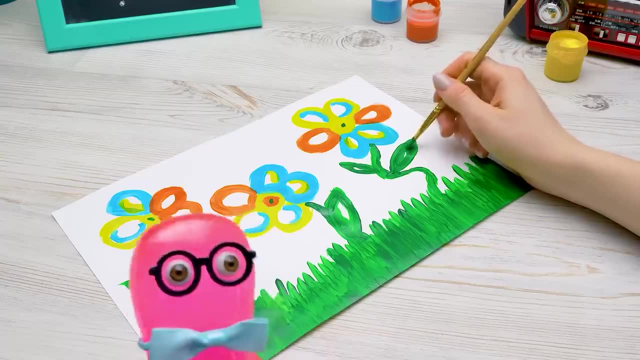 Oh, I thought you were my purple cow. That's true, I am the best, But the ideas also need to be unique, And then we'll take over the world. Let's go, I'll show you Cool. Oh boy guys, something is coming. 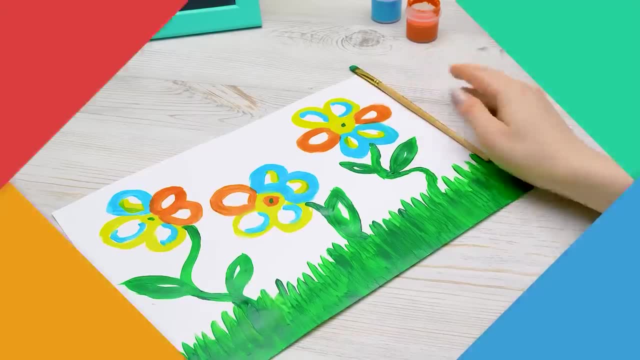 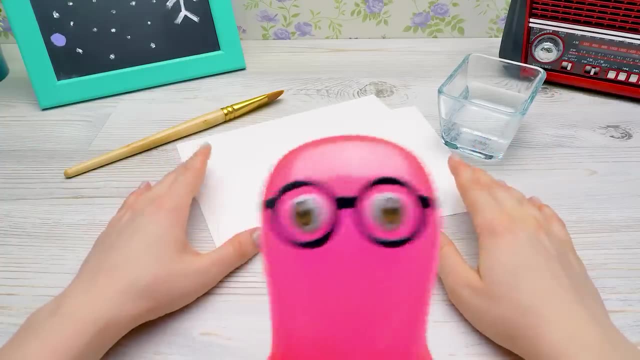 Command marketing genius. What do you need? Hmm, Let me see. Thick drawing paper is here. A brush Here. Water, Here we go. Hmm, And food coloring. I hope you won't eat it, No, No. 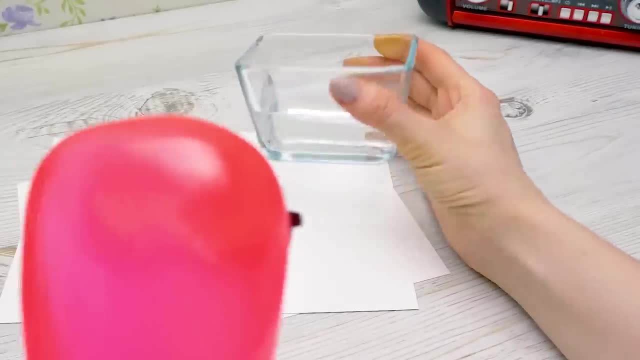 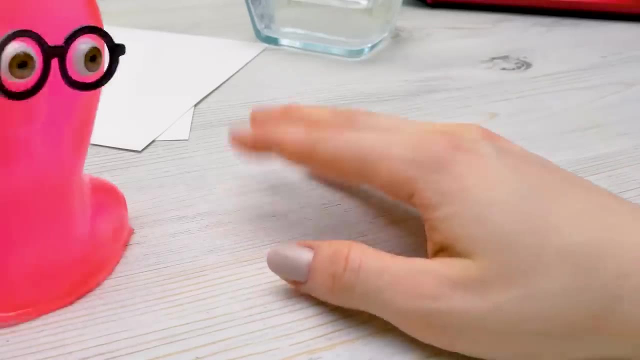 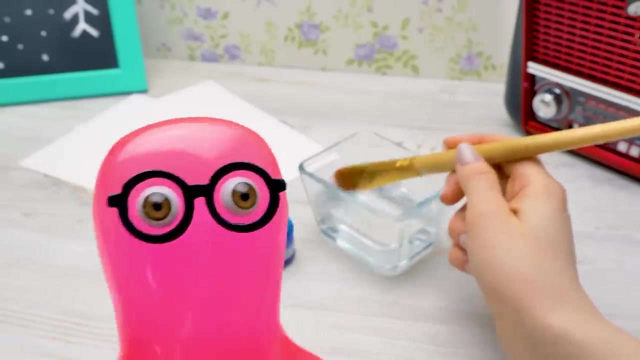 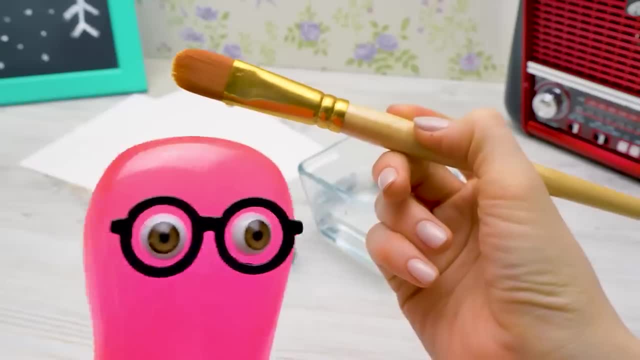 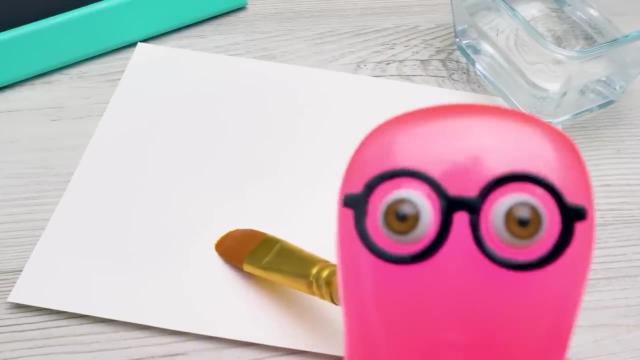 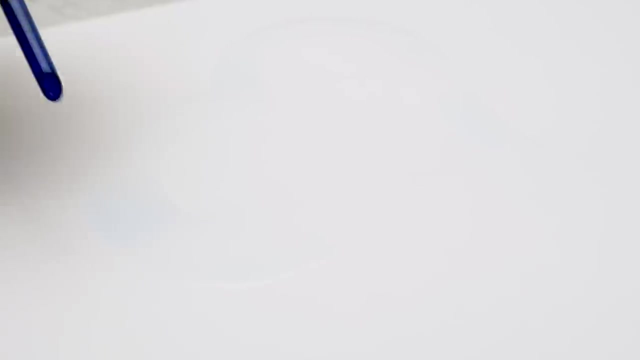 Dear viewers, I urge you to try this at home. Maestro, Ahem, Uh, Sam, are you sure about this? Sh مشh, Now Get some food coloring and drop it little by little. Heh Ha-ha. 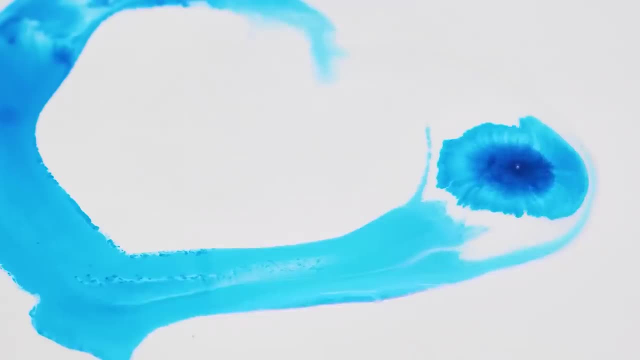 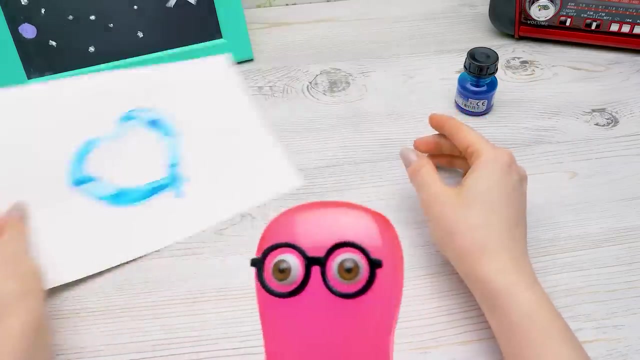 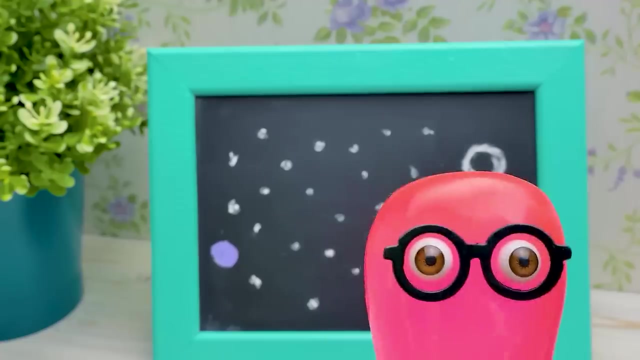 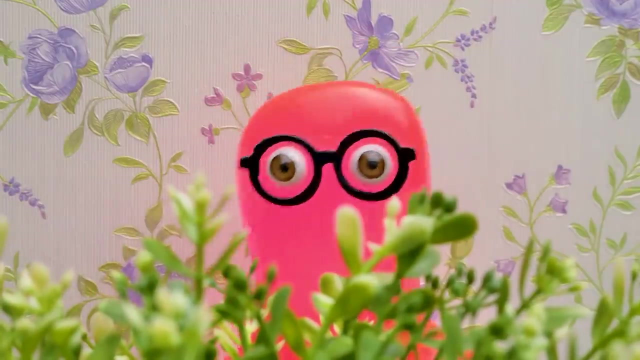 Wow, Sammy, you should do drawing workshops Exactly. How did I not think of it myself? Oh, I know so much, I draw so well, And they won't let me pay for candy with my smile. It's done, I'm doing an art workshop. 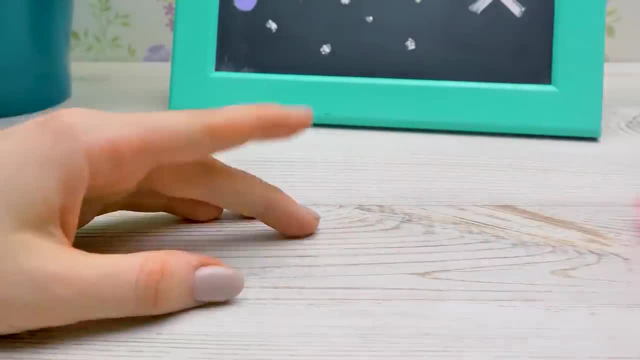 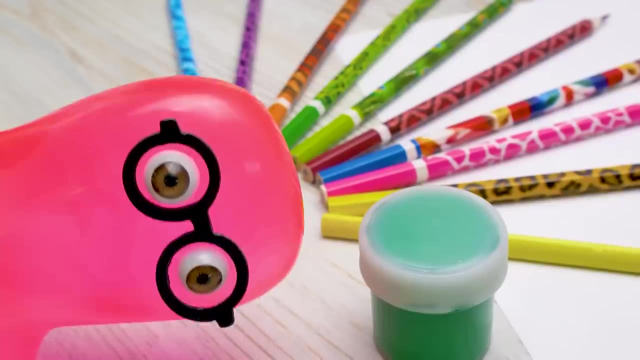 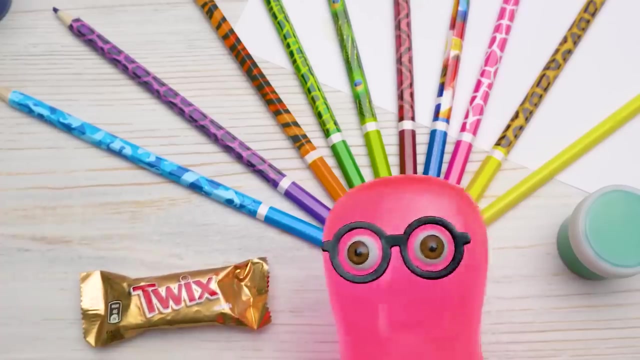 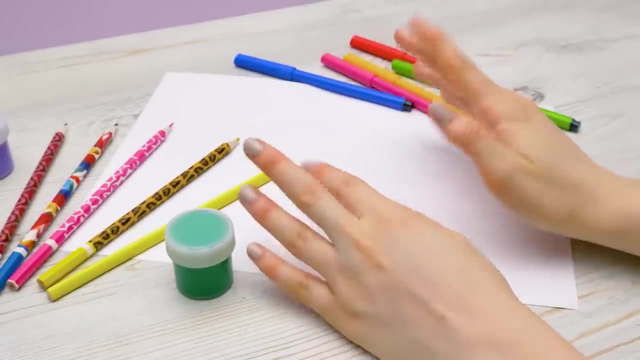 Yay, High-five. Uh yeah, okay, we'll work on it. Nobody called and it's been a whole day. Sammy, look, Candy, Candy, Susan. Life is suffering, Disrecognized, Unwanted genius. Are you sure the phone number is right? 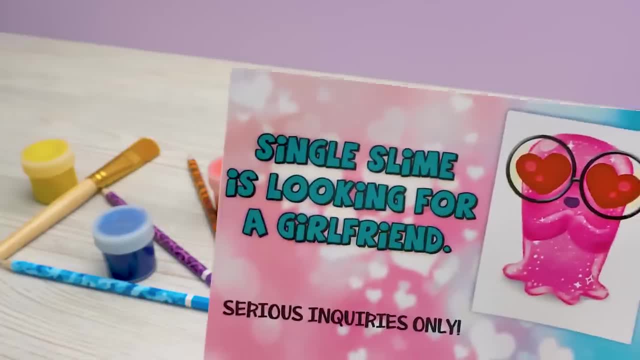 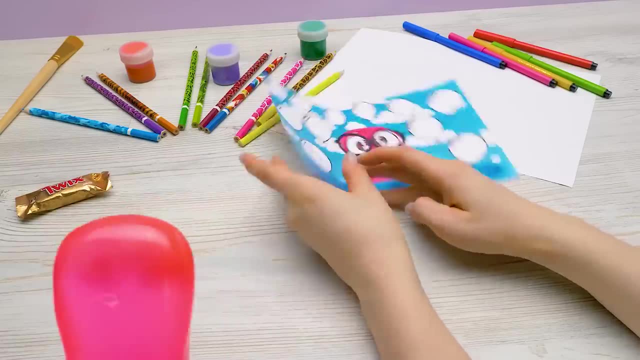 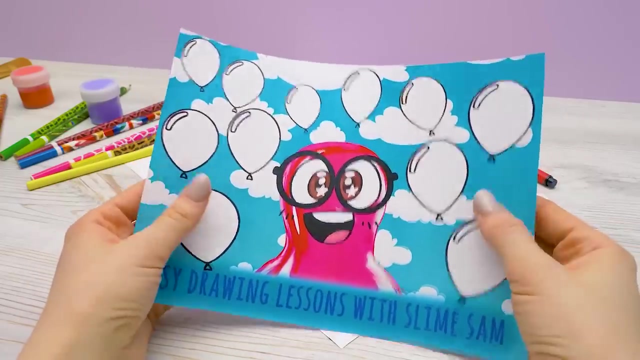 Of course I'm sure. Well, show me your ad Here, Huh, Oh no, that's not it. This one, Sammy. no offense, but it looks nothing like a purple cow. You lost me. You told me yourself that to be noticed, you need to stand out. 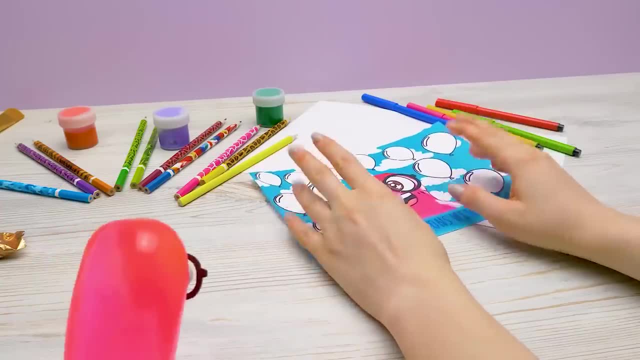 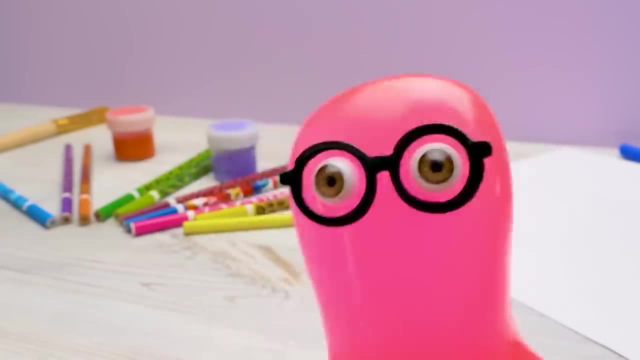 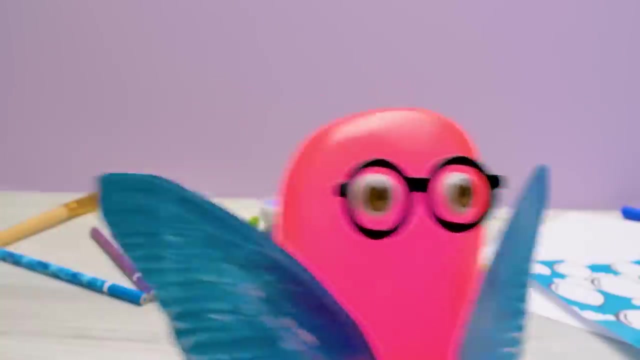 Yeah, Can you imagine how many people sell drawing lessons? You need a thing, Something that nobody else does. I can sing during the lessons. I believe I can fly, I believe I can, I believe I can touch the sky. No, a drawing thing, I think. 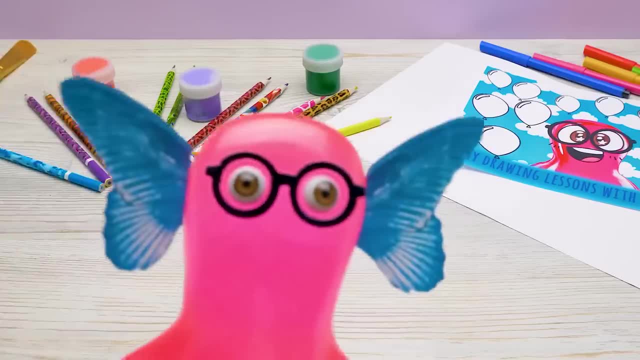 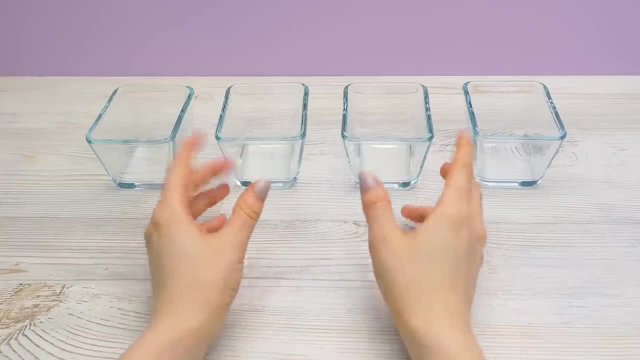 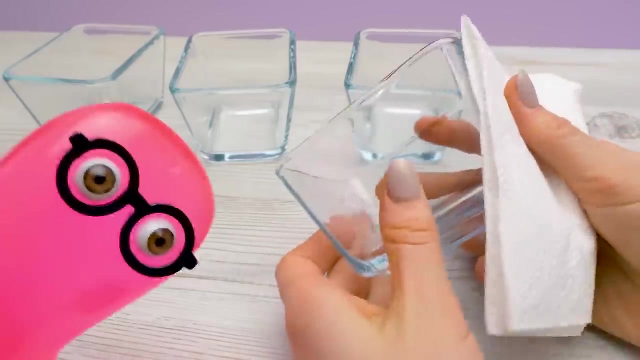 I have an idea: Fast, fast. I can't wait to start teaching. Do you remember how we made fluffy slime? I'll say the best snooze of my life. Puppy slime paint will be your thing, I'm ready. We'll need fluffy slime ingredients except for: 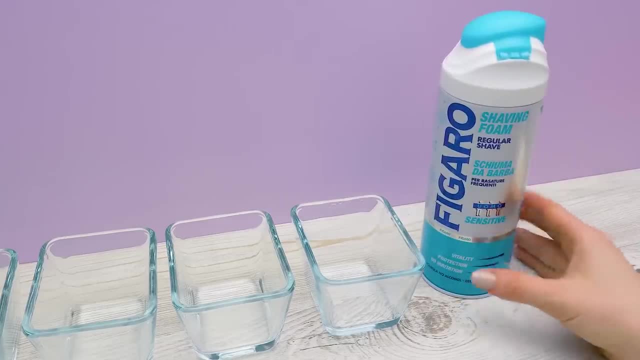 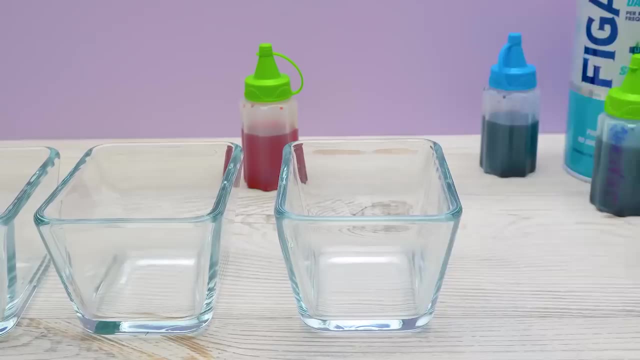 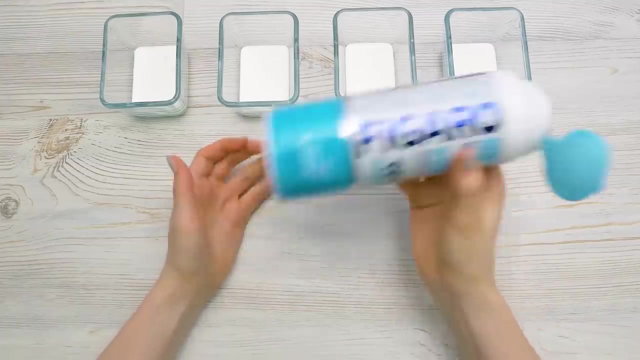 Oops, White glue, Shaving cream, Food coloring And a few bowls for the different colors. First I'll pour the glue into the bowls like this. Now I'll add shaving cream to each bowl. Hmm, I think I better fill it up to the top, like this: 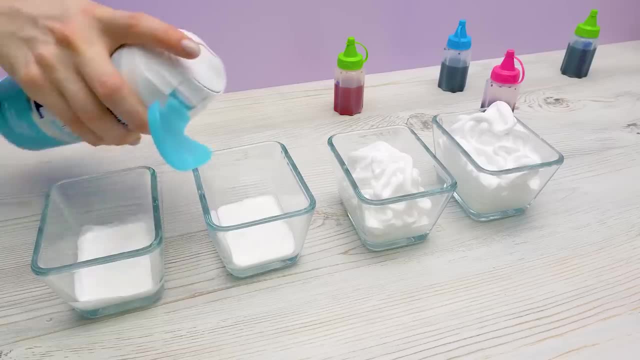 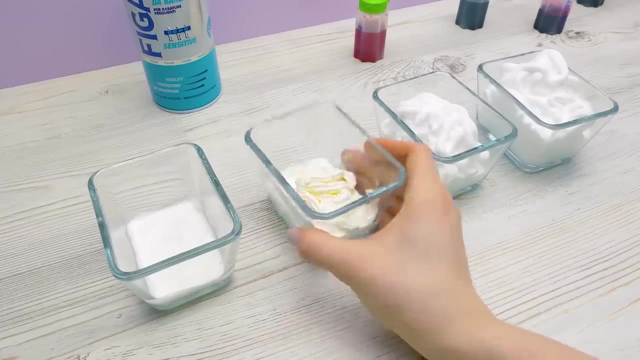 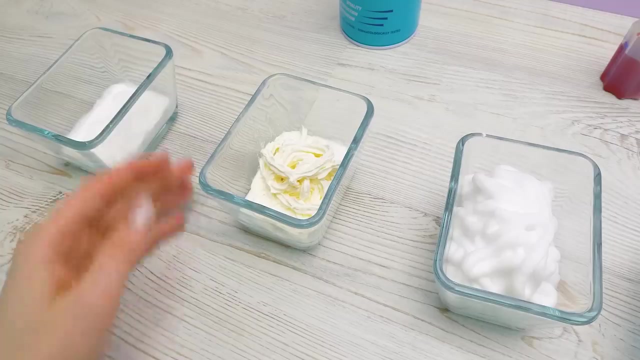 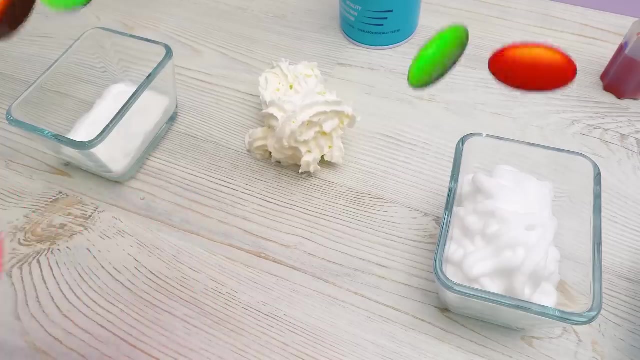 And the same amount here And Ready, Aim Fire. Woo-hoo, Woo-hoo, Woo-hoo. Oh Sam, That's whipped cream. Sweet Sammy needs sweet paint. Okay, one color less. We'll see about that. 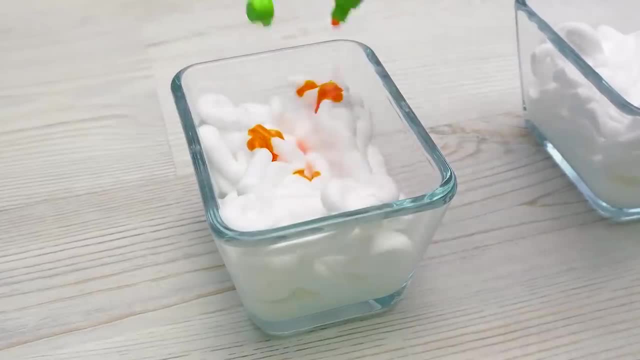 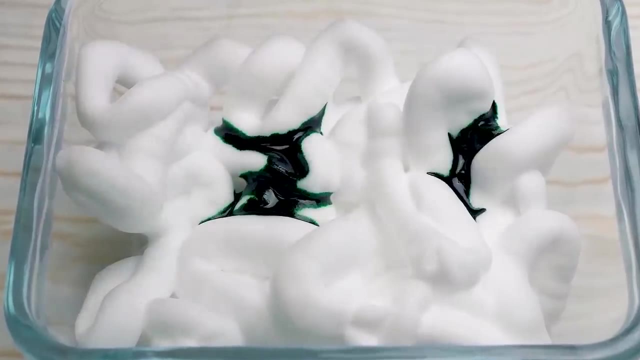 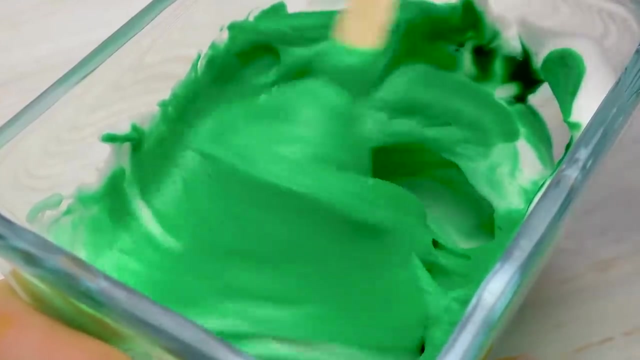 The last step is to add food coloring And stir. The color is so intense, Don't overdo it. Don't overdo it, guys, And one And two, And one, Two, Three, Ugggggh Sugar. 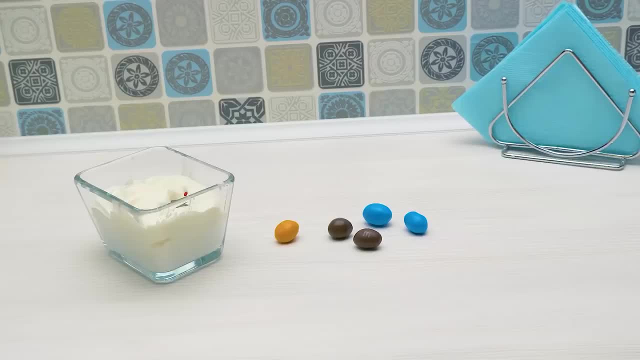 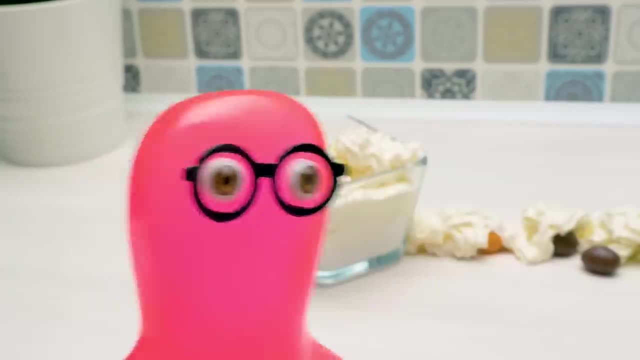 Yes, please, It could never be too much for me. I'm right here, Cause I need Little candy, little sympathy. Oh Sweet, little candy, little sympathy. All right, What do you call that, Honey, Honey. 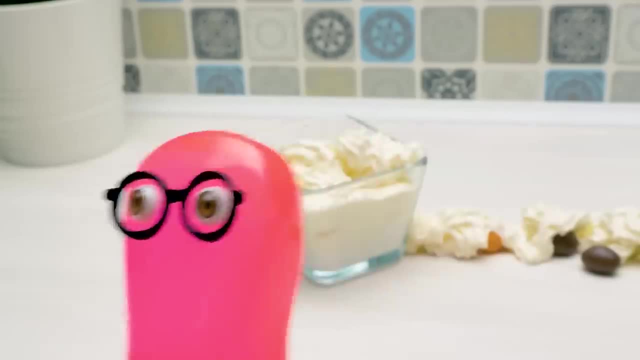 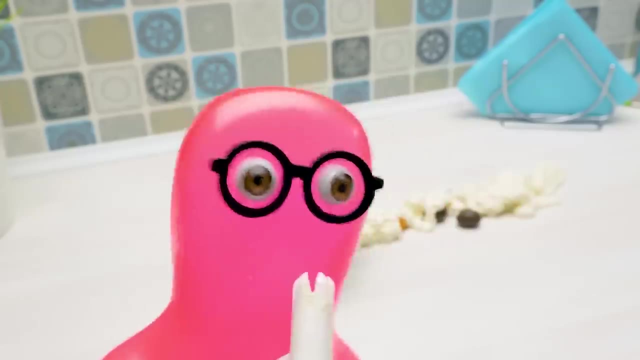 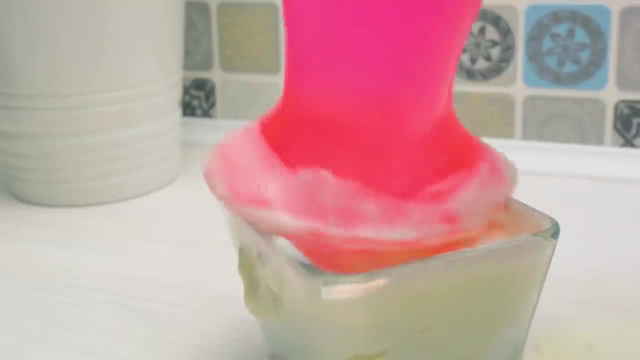 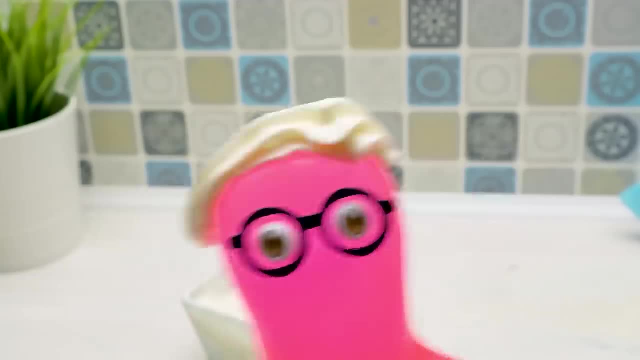 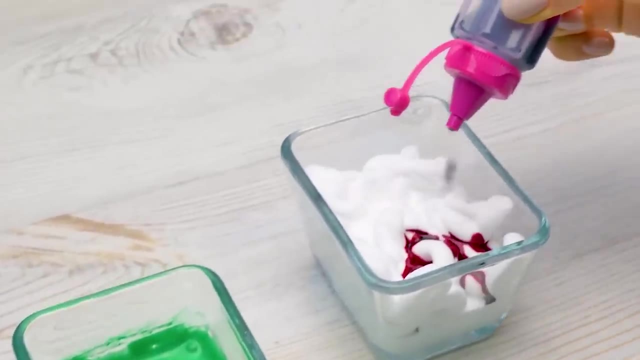 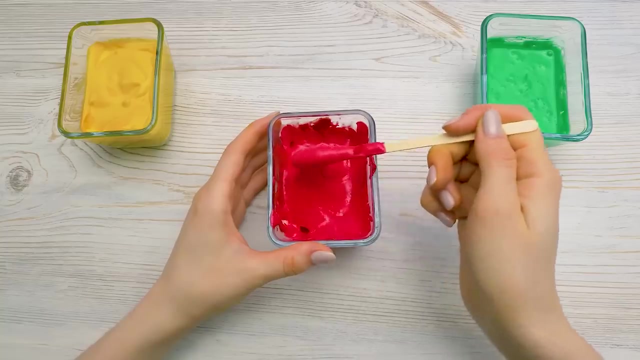 Sugar. Yes, please, It could never be too much for me. Almost done here. Just one more color. It looks pretty cool so far, guys. Look at this texture. Guys, what do you think these paints look like? Comment below. 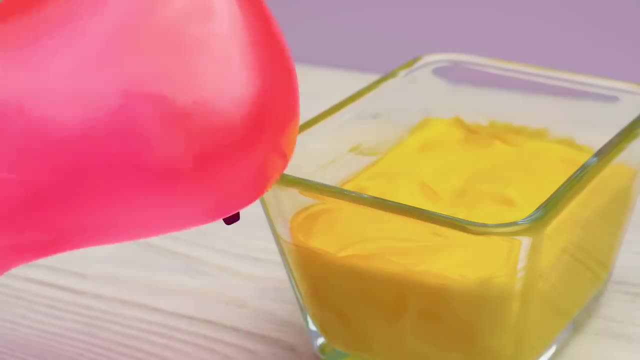 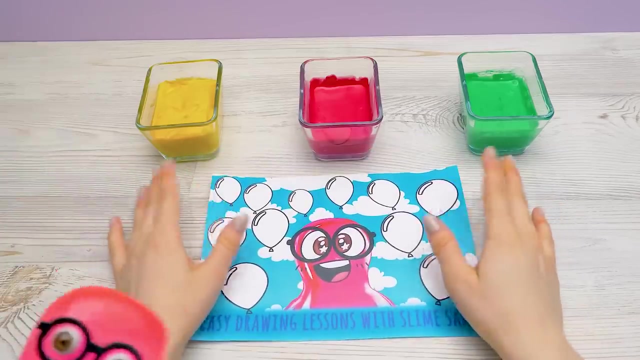 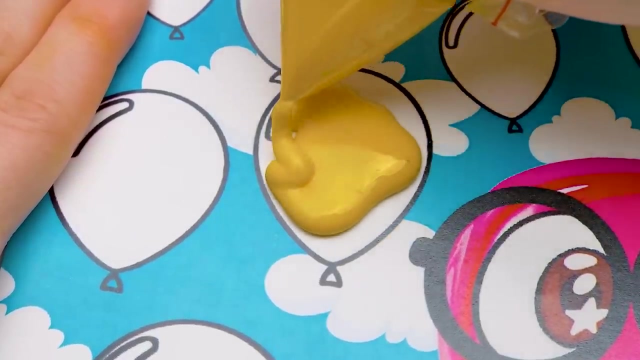 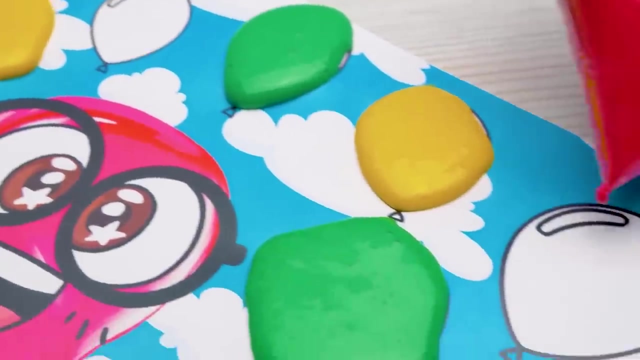 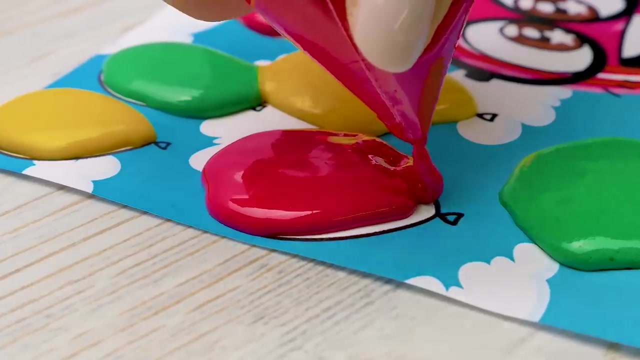 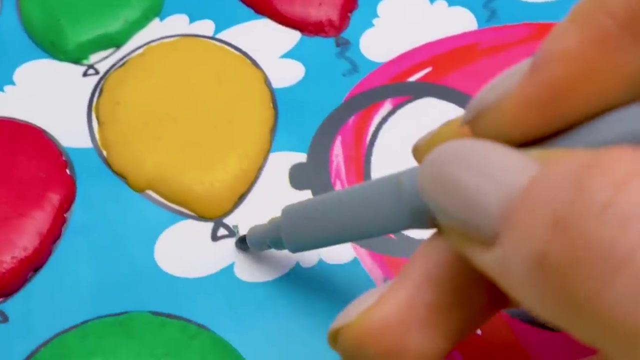 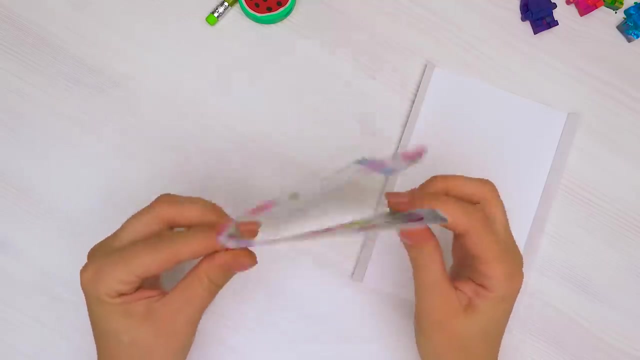 Oh, is that them? It's them, Sam. They are so fluffy. How about we try and improve your ad? Yes, please, I'll start making the next drawing. To add more magic to it, we'll need the following things. 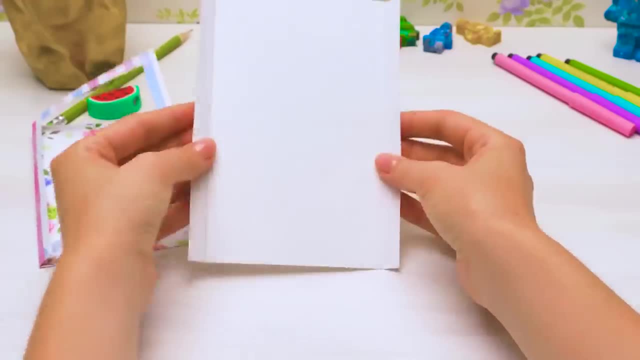 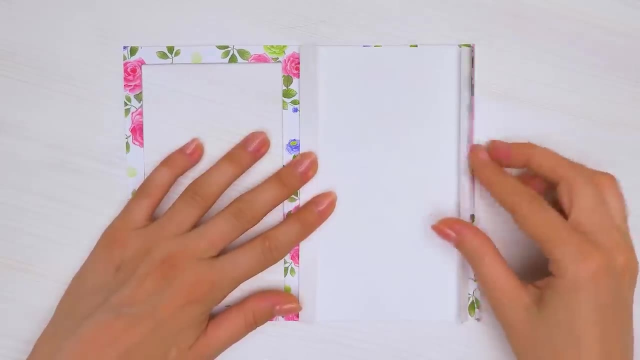 I've prepared this paper frame in advance And this piece of paper to fit in Where we need to fold the sides in. Let's do it. Let's do it Like this: Now, let's check. The paper should be hidden in the frame perfectly. 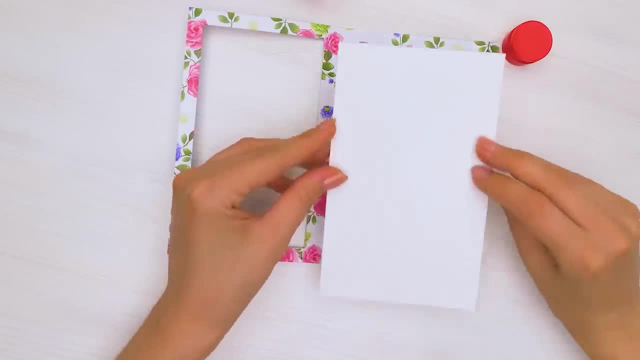 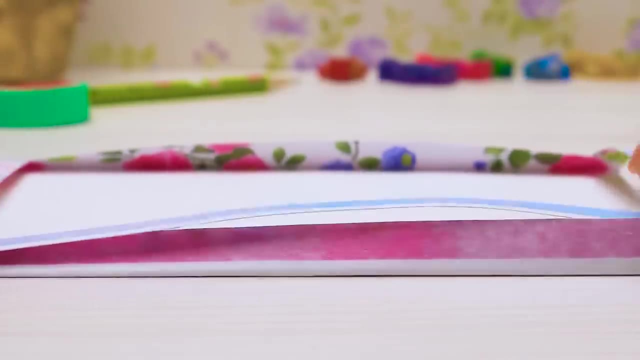 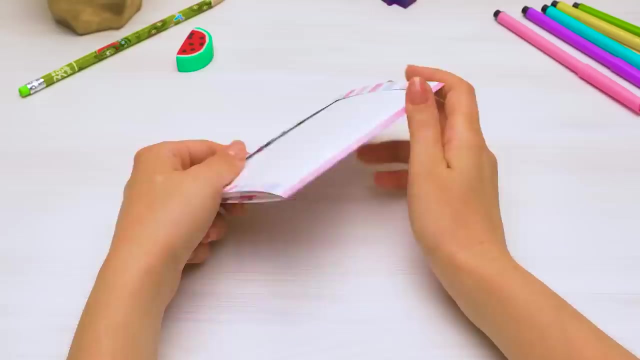 Great, Now I'll apply some glue and stick it inside. Let's apply some glue to the frame as well And seal it, So one part is ready. For the next step, I'm going to need a piece of paper to fit into the frame. 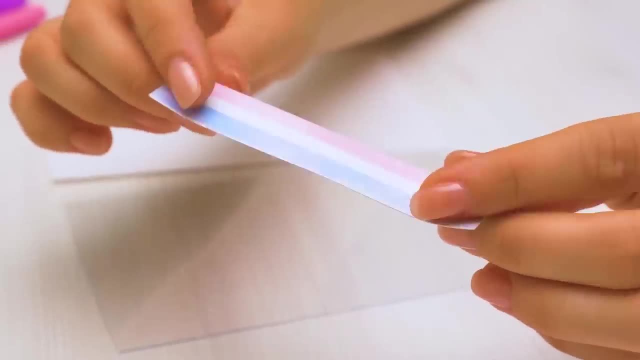 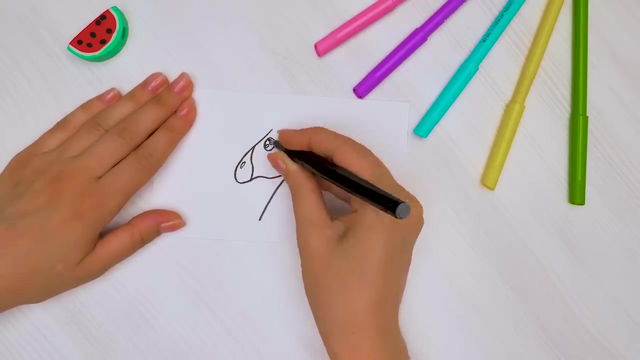 and transparent film or thin plexiglass And a small rectangle from the same piece of paper as our frame. I'll draw a unicorn on the white paper. Oh, I love drawing magical creatures, Do you guys? Next, I'll color it brightly. 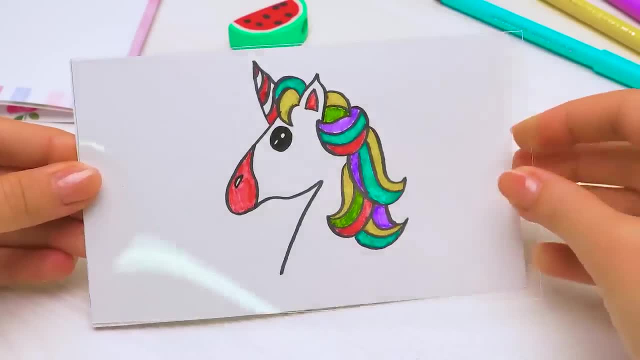 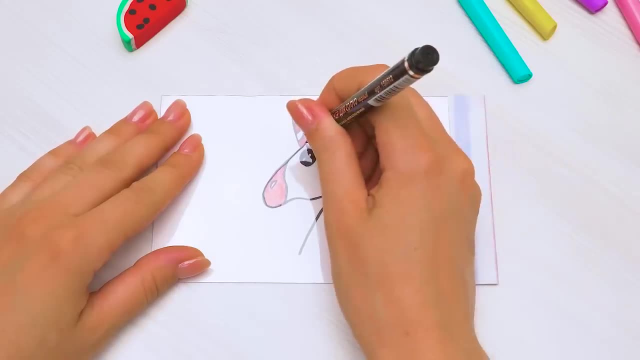 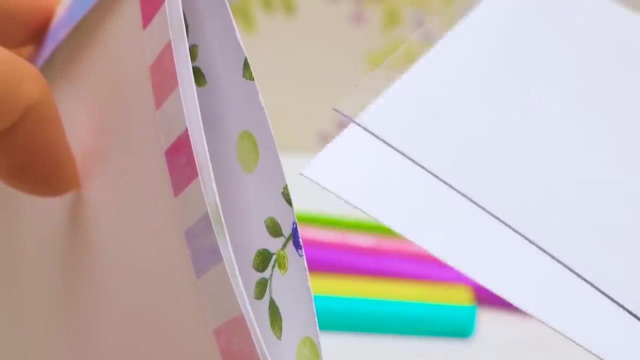 Now we'll place the film onto the drawing and glue the rectangle to one side, Right. let's move on to our trick. We'll outline the drawing on top of the film. It'll create an amazing effect. Now we can connect our parts. 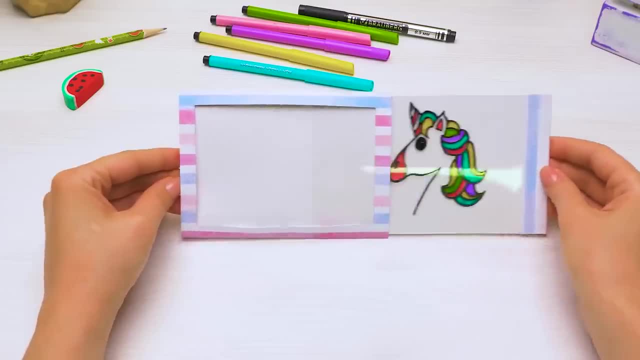 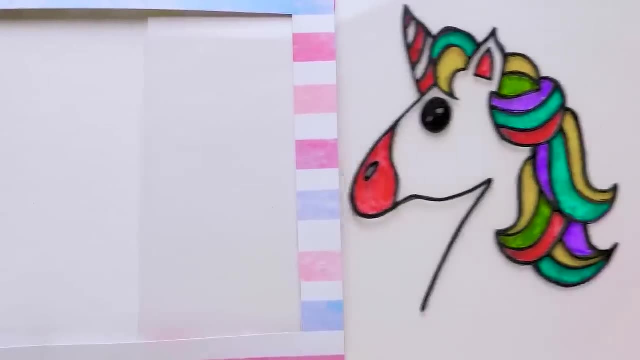 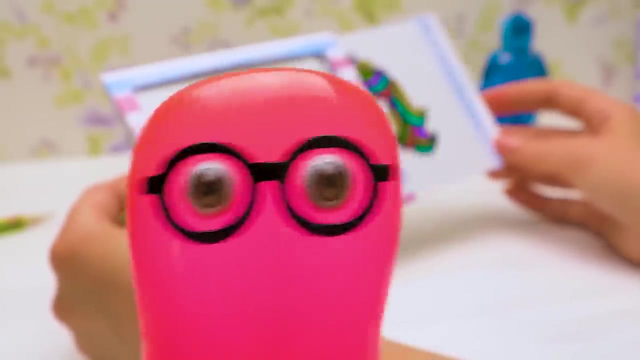 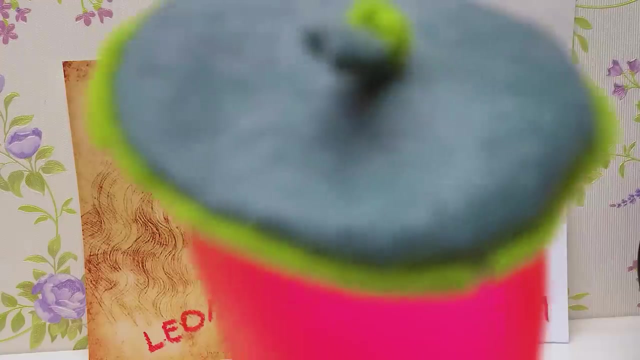 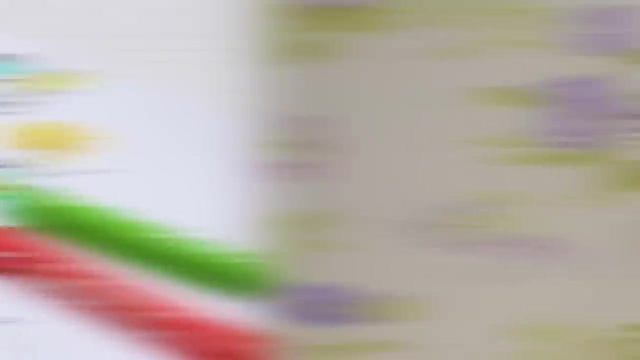 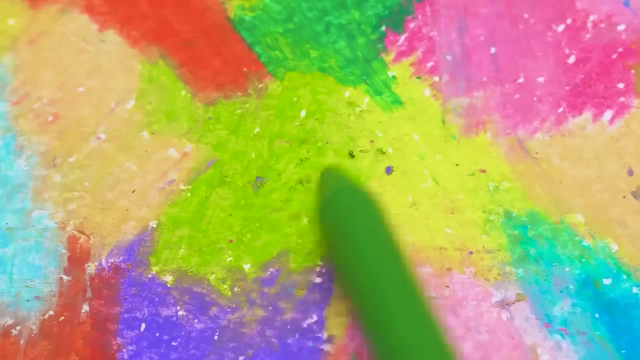 Like this. Wow guys, look, It's real magic. Wow, A unicorn, Suzy, can I play with it? Can I, can I? can I Sure Sam Here? Yahoo, Wahoo, Right, I need to here and here. 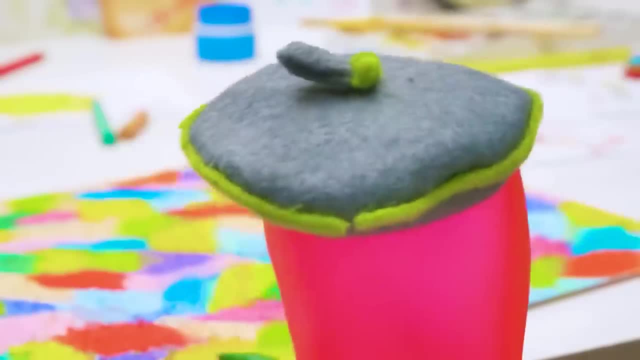 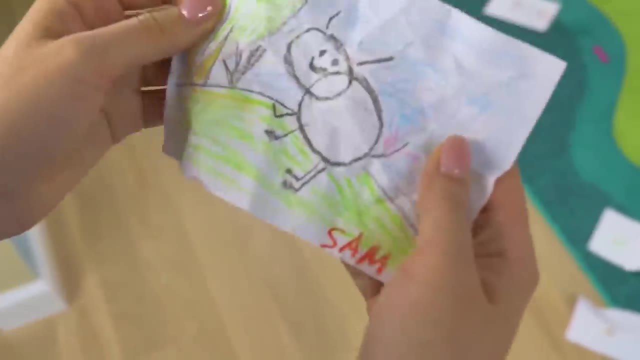 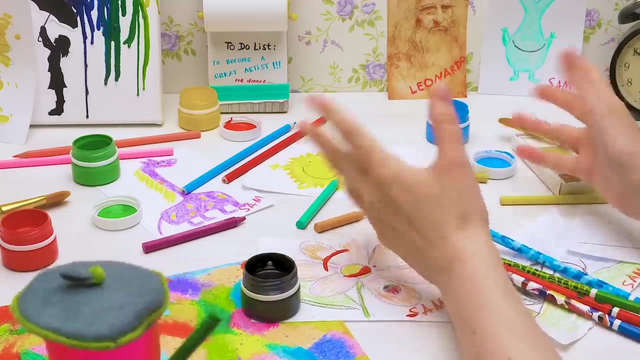 Oh, drawing is no simple task, Right here and here. Hmm, what's this, Sam? what's all this mess? Do you really need all this? Pencils, pastels, paints, Hi, What are you doing? 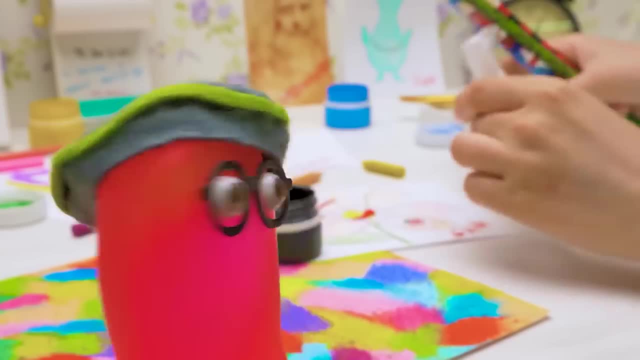 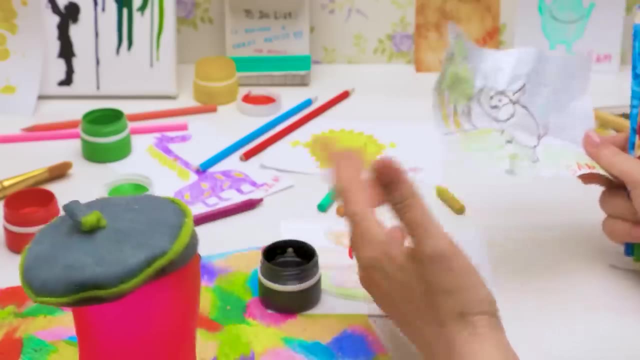 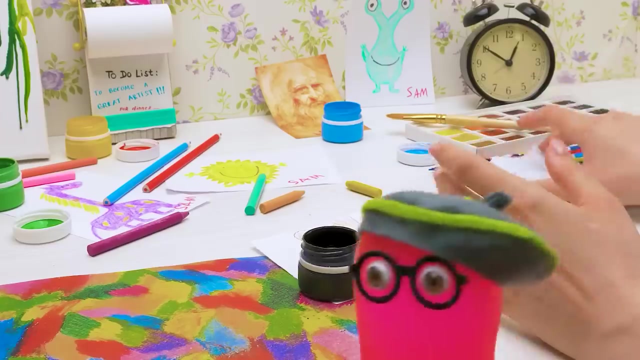 Trying to figure out what you're doing, As if you can't tell, I'm creating masterpieces. Oh, I see, Sue put that down. It's a sketch of my future masterpiece canvas. You didn't say please, Oh, please, Sue, don't get in the way of my masterpiece. Please leave, Come on. 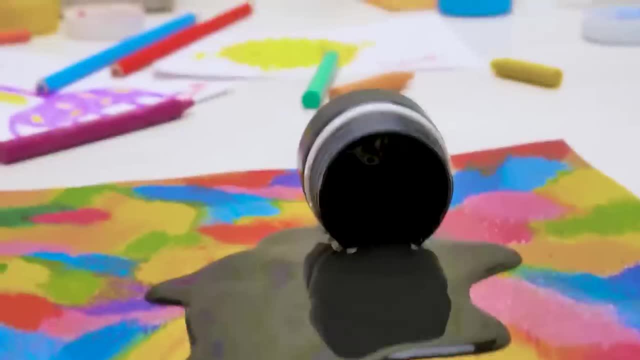 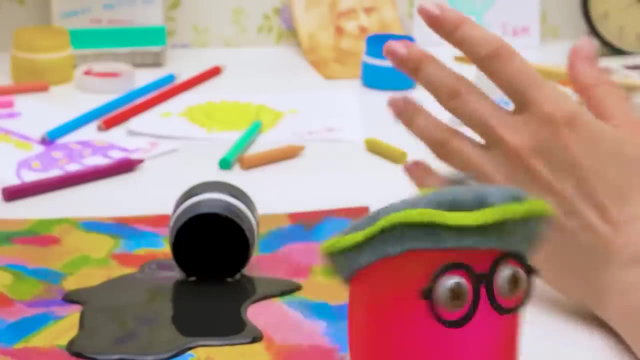 Well alright. Oh no, It's ruined. No, It's horrible. Oh, that's a catastrophe, Sue, how could you? Oh, I'm so sorry, Sammy, It was an accident, but you can paint a new one, right. 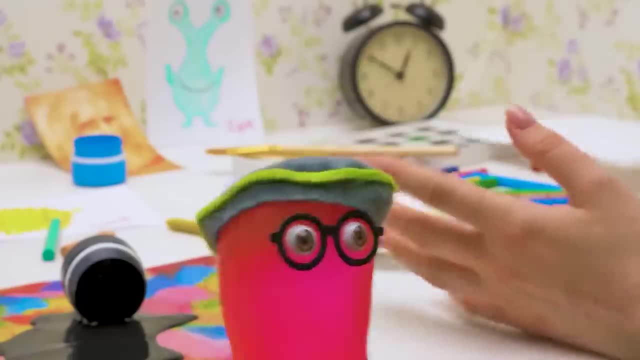 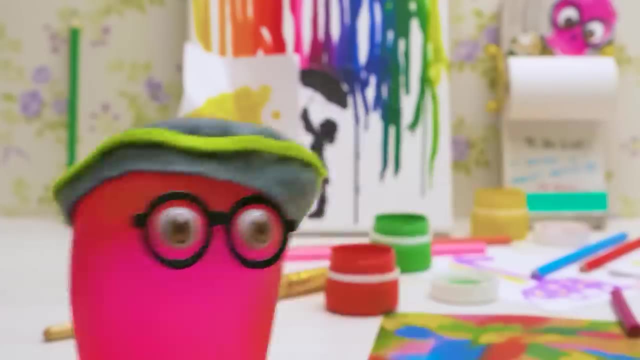 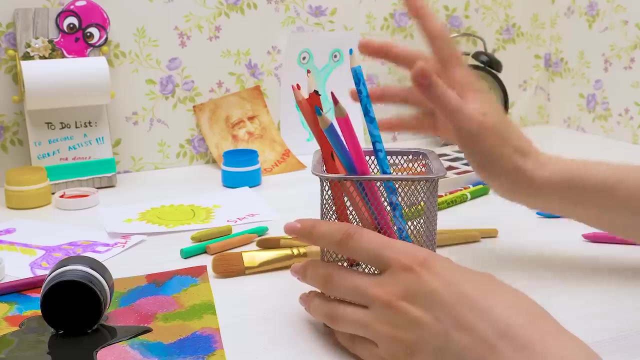 After all this, No, My inspiration is stolen. Now all I can see is eternal creative crisis and oblivion. Hi guys, Oh, what did you do? Oh, no, Sammy is so upset. I need to think of a way to get Sam's inspiration back and quick. 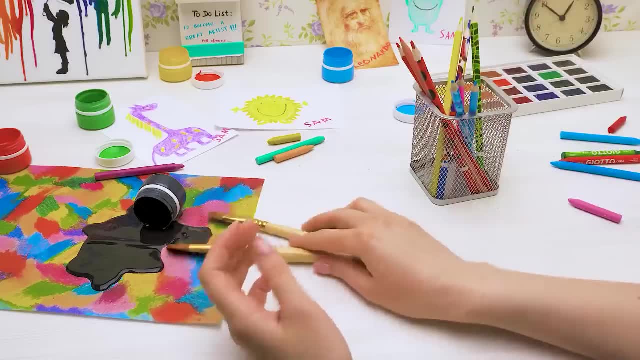 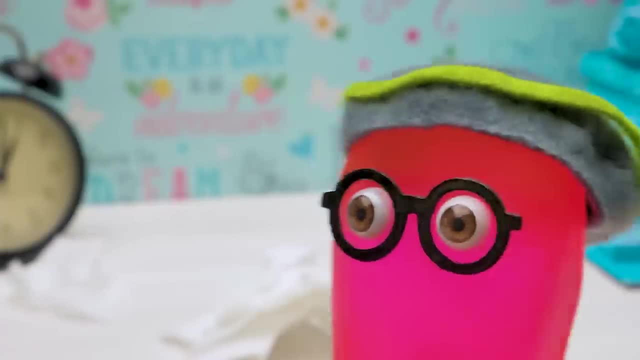 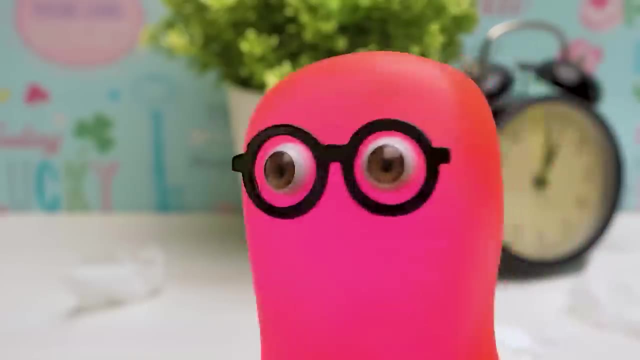 What inspires you? Comment below, Perhaps something will be good for Sam. Oh, I have an idea: My career as an artist finished before it even begun. Nobody will need me now, Guys, maybe you still need me. Could you subscribe, please and hit the bell button. It might comfort me. 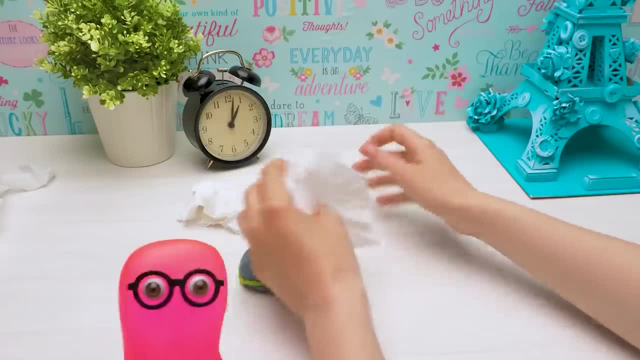 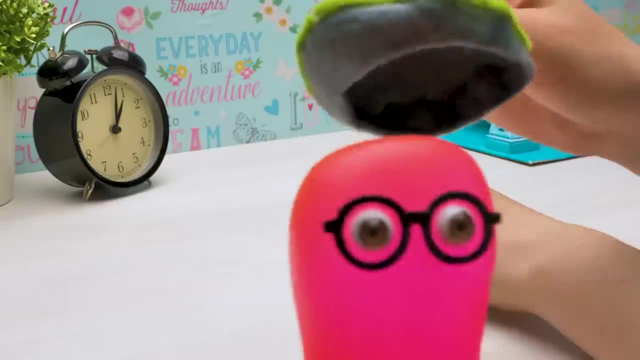 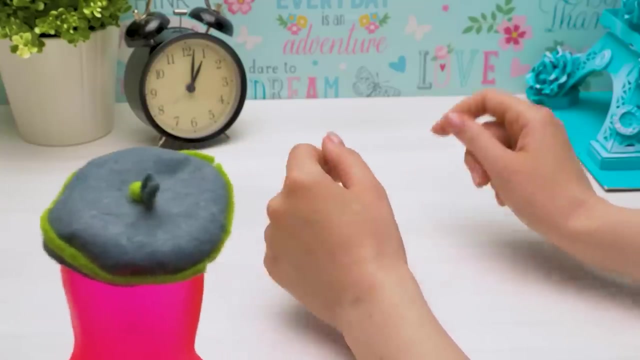 Sammy, I know what else can comfort you. Oh, you again Came to ruin something else. No, no, I know one way that can still inspire you and bring your artistic skill to the next level. There is no way to do it. You spilled black paint all over my artistic talent. 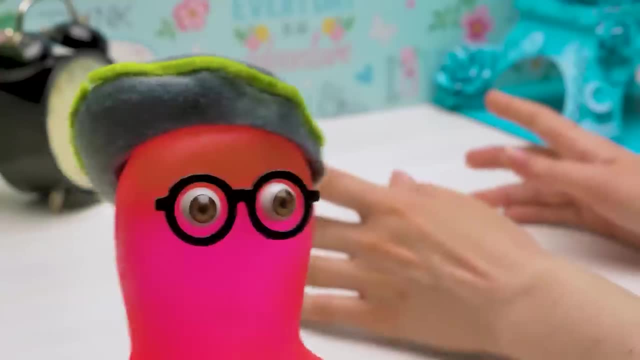 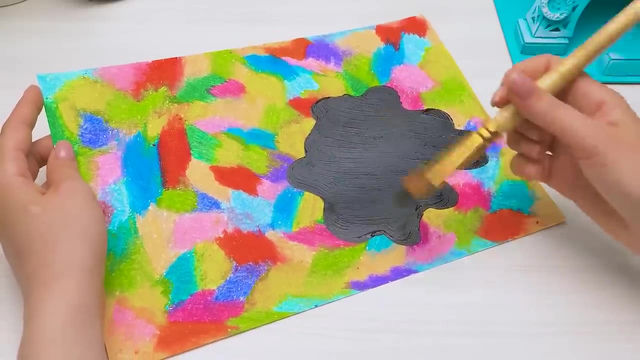 There is Sammy. Please give me a chance. Hmm, Well, alright, I'll give you one more chance, Thank you. First, let's complete the process of covering your drawing with black paint. Oh no, I want you to stop it. 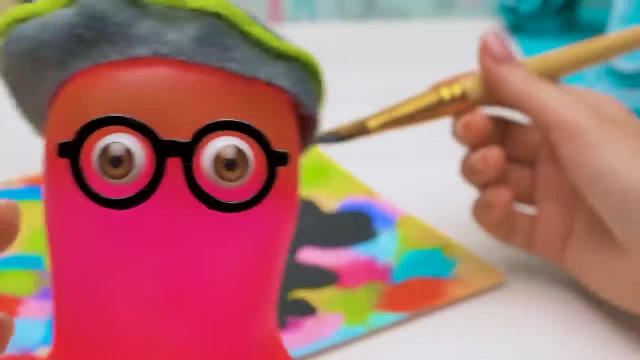 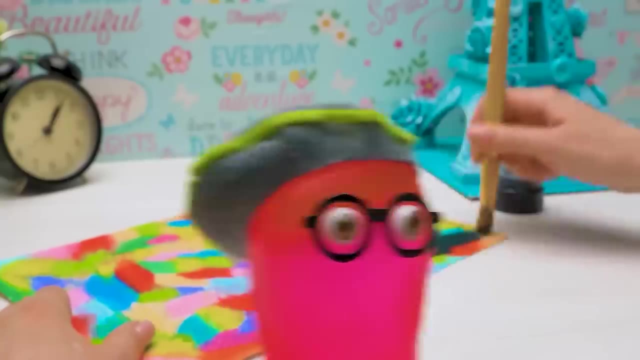 Sammy, it's okay, Calm down, Everything will be alright. Oh well, fine, We need to cover the whole paper evenly. Oh no, I can't watch. Sue, are you sure you're alright and you're not trying to create Malevich's rectangle? 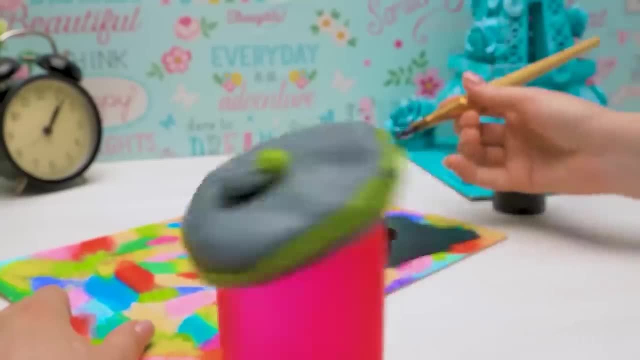 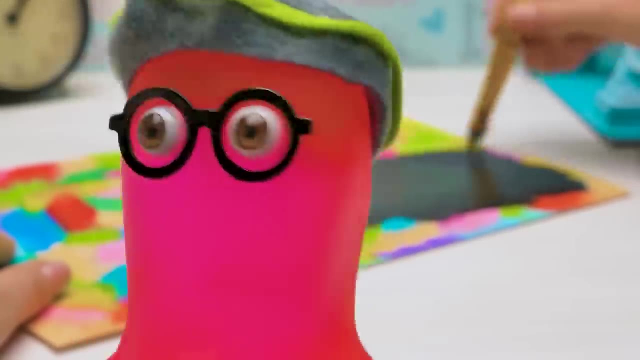 Square, Sammy, A what Malevich's square? Uh, but it's a rectangle. Really, Sue, you don't seem right in the head today. No, Sam, it's the name of the painting: Malevich's square. 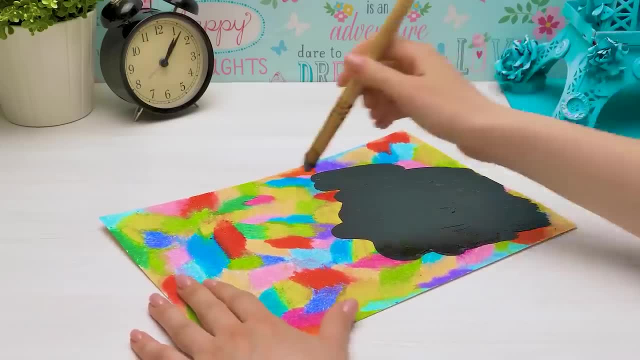 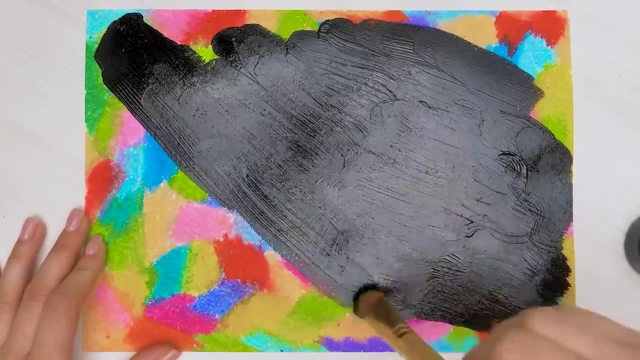 Sam, it's the name of the painting: Malevich's black square. But I'm making something different. Oh, now I'm starting to get it. Yeah, no, no, I don't get it. You'll see soon enough. It's pretty magical. 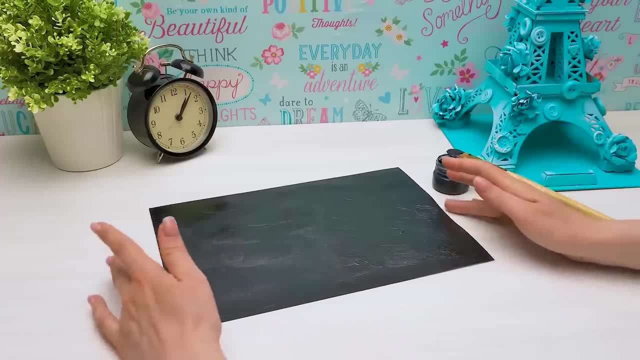 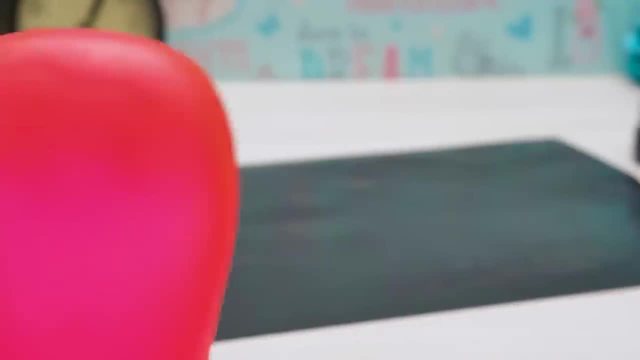 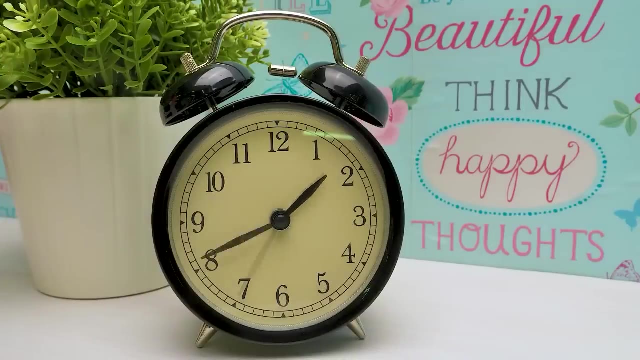 Alright, the paper is completely covered with paint, so now we need to dry it. I'm coming, coming, I'll dry faster. Come on, Sam, maybe we just need to leave the paper alone. Oh fine, Done, Sammy, The paint is dry.